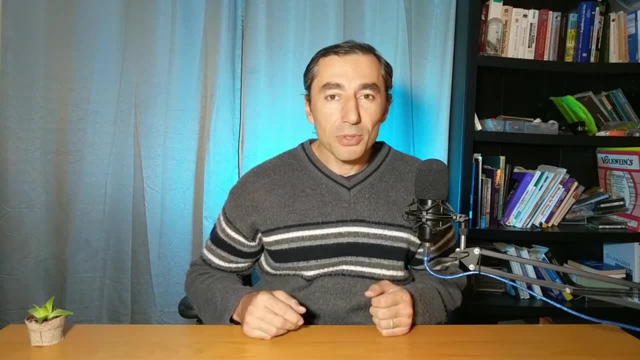 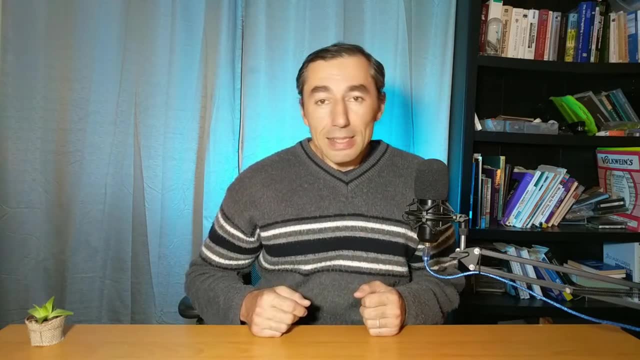 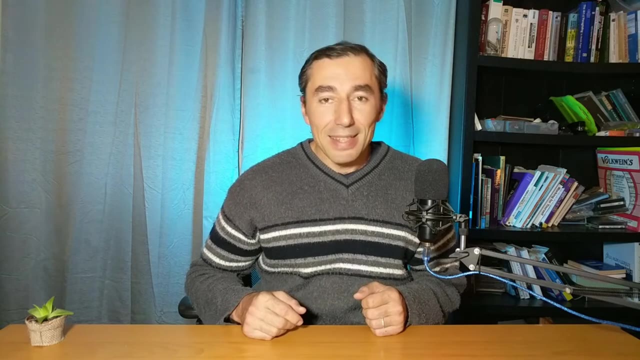 using your typical data structures, such as hash maps, trees and so forth, you probably notice that things get ugly quite quickly, in particular when needing to merge two groups together. this is because, inevitably, you have to copy every user one by one, which results in order and running time. now let's see how. 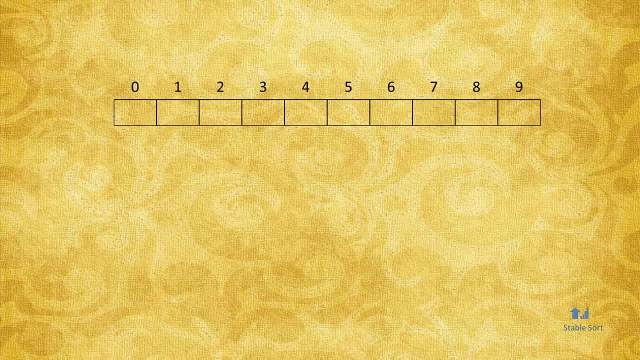 this joint set comes to the rescue. amazingly, all that's required to solve this problem is a simple integer array. we're going to assume that user IDs are positive integers and will allocate an array to hold all of the IDs. so if there are n users, we create an array of size. 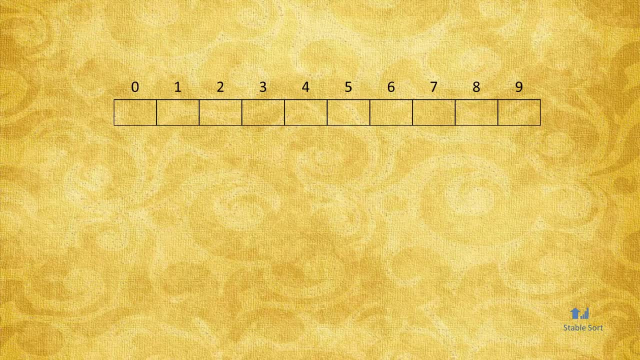 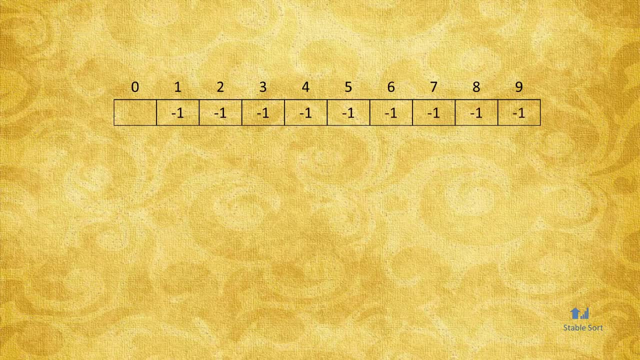 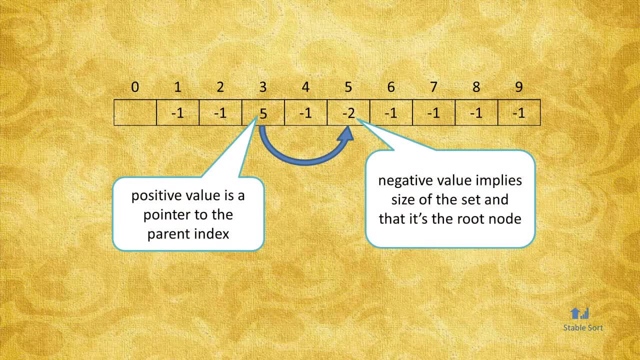 5. we store the size of the group. in this case, since there are only two users involved, we want to store the value of 2, except we'll store the negative value, negative 2 in this case, to be able to tell apart a group size versus a. 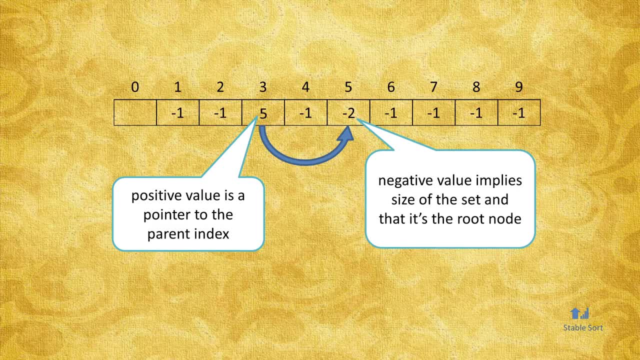 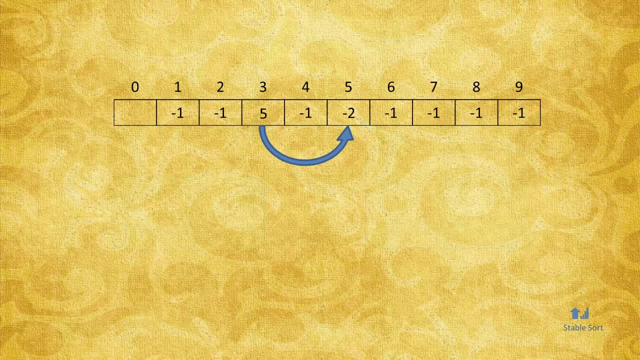 reference to some other index. so a positive value is like a pointer to the parent index, while a negative value signifies the size of the group. let's continue with this example. suppose now user 6 becomes friends with user 3, so we'll set 3 into the array at index 6. then we'll look up at the value at index. 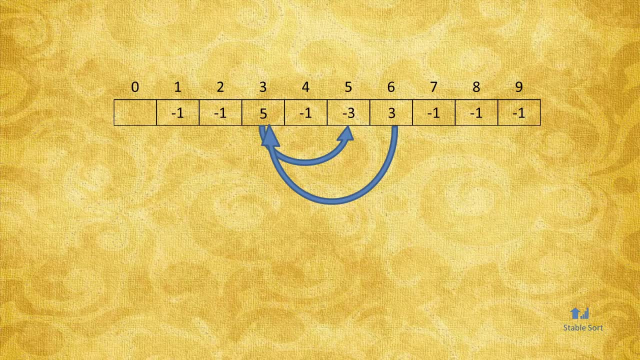 3 and since it's positive, we know that this is a pointer. so we follow the pointer to look at the value at index 5. there the value is negative. so this must be the end of the chain. and we're looking at the size of the group. we increment the size to 3 and again store. 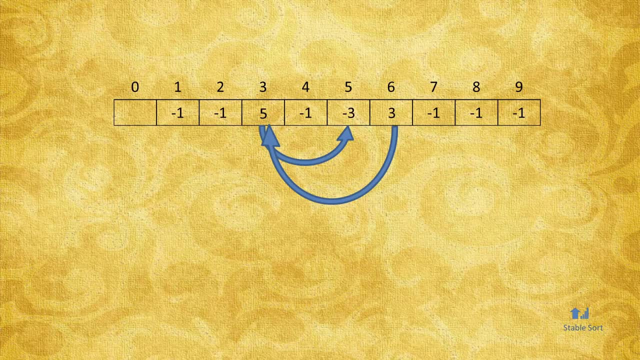 the negative of it. since these path chains can get long, one of the musician that we could make is to link directly to the end of the chain, thus keeping the path as short as possible. this optimization is called path compression. here's another example where two groups are being merged into one.